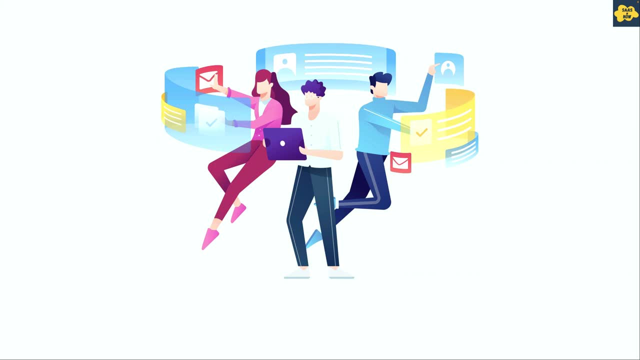 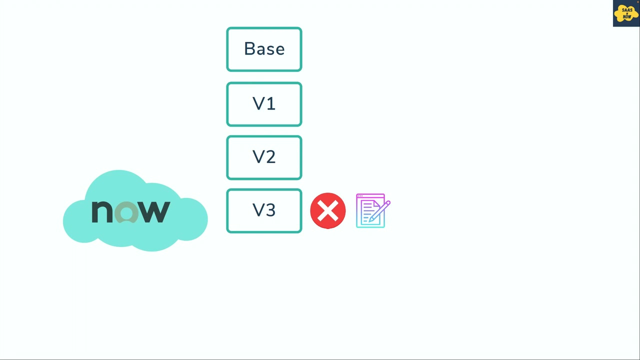 Technical teams started the investigation. Teams started validating if there was a requirement to change this functionality in last release and they found that there was no requirement to change this existing feature in last release. However, a developer broke this existing feature while working on some other. 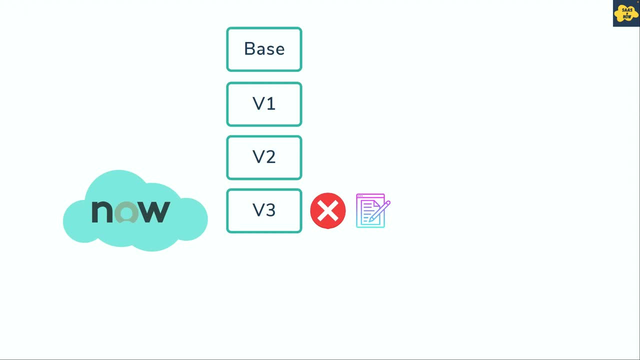 unrelated requirements, Which was part of last release. Team also validated that testing was performed in last release but still exists. functionality got broken. Now the question is: did testing team perform testing of previous changes done before last lease? and the answer was no, and This is the reason due to which broken functionality. 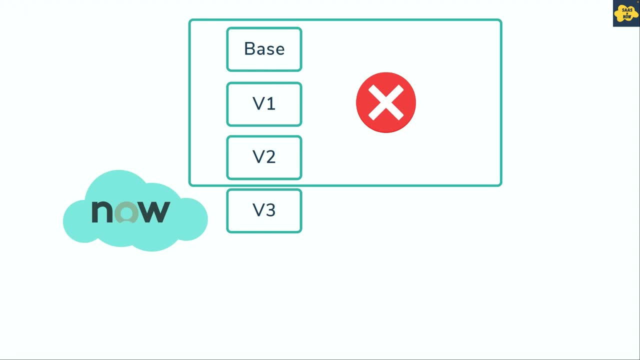 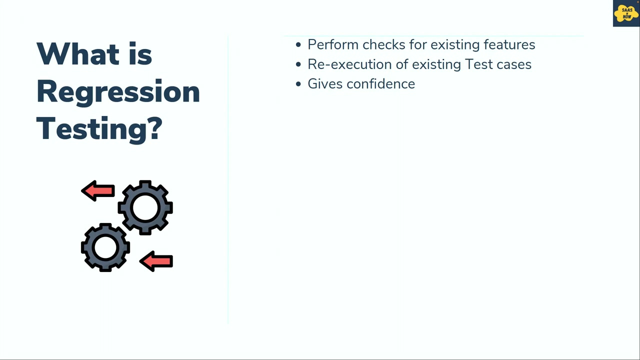 was not caught during testing of the release. So basically, it is recommended to test existing functionalities before new production release to make sure existing functionality is not broken, and this is called regression testing. So regression testing is a type of software testing to perform checks for existing features if they are working as 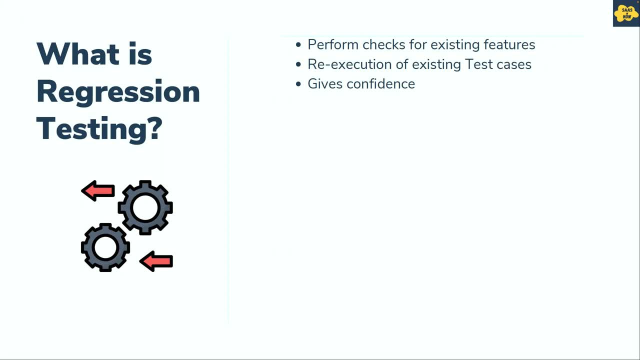 expected After recent development changes. it is re-execution of existing test cases created for existing features to ensure existing functionalities are working fine. It gives confidence to developers, testers, stakeholders that there is no existing functionality broken after production change. Now why we do regression testing. 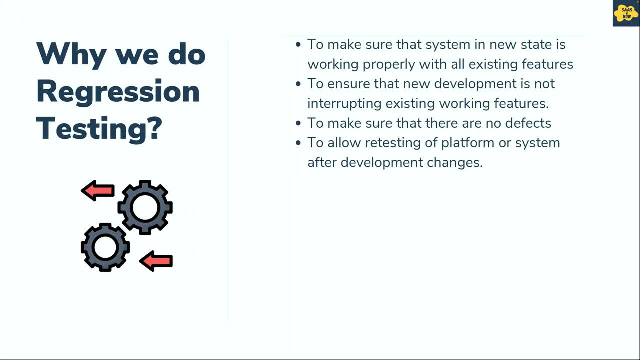 Sometimes other parts of the system can behave unexpectedly due to new modifications, which means features which used to work got some bugs. So testing team needs to make sure that system in new state is working properly with all existing features, and that is why regression comes into the picture. 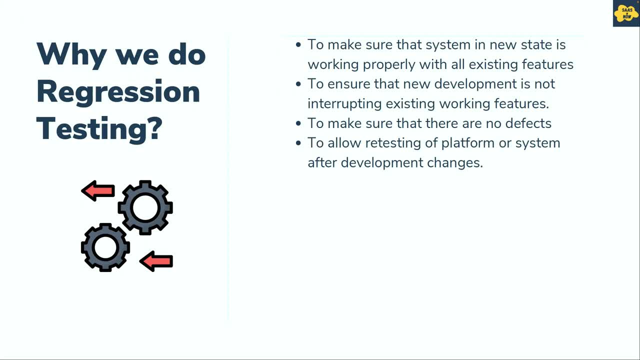 Regression ensures that new development is not interrupting existing working features. We need to do regression to make sure that there are no defects or bugs after implementing new development changes. We do regression to allow retesting of the platform or system after development changes. Now, when do we do regression testing? 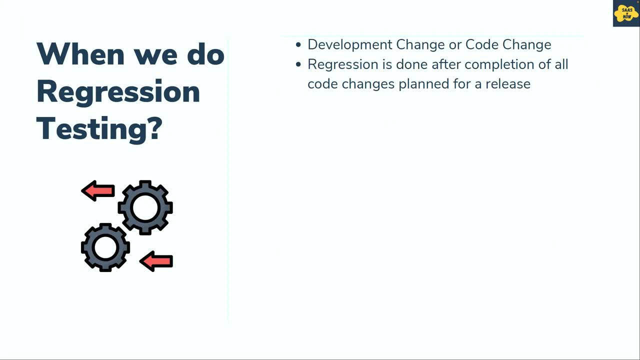 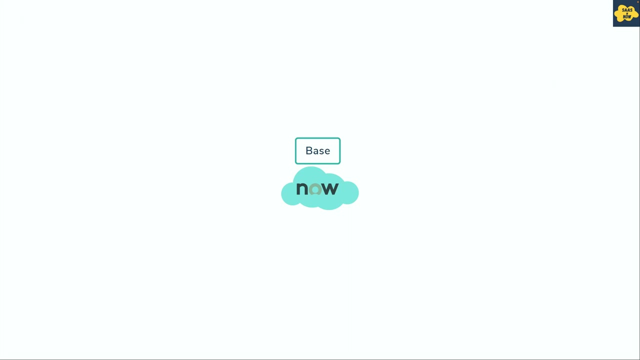 We do regression testing when there is any development change or code change in the platform which could be a new feature, enhancement or bug fix. Regression testing is performed after completion of all changes planned for a particular release. Let's understand this with an example. You have a ServiceNow system with out-of-the-box baseline features. 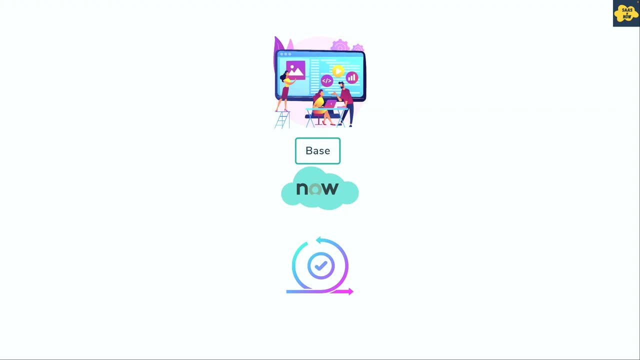 which are working features. Testing team creates test cases for different scenarios for existing functionalities and features. Let's say there is a new requirement from a customer to make a field mandatory on incident form in ServiceNow. platform Development team will follow a release path in which requirement will be developed. 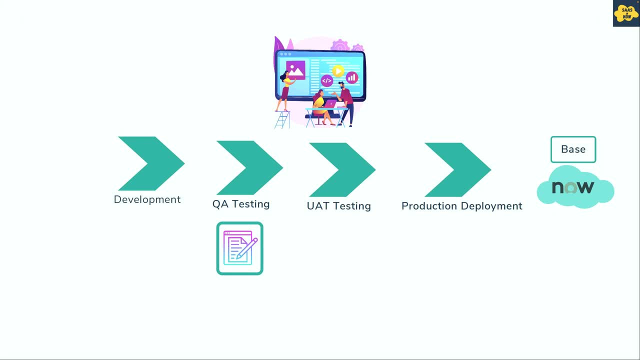 Then it will go for QA testing And then Testing team will perform regression testing to make sure that new requirement has not broken any other feature of the platform. After regression, UAT testing is done for that particular new requirement, that new feature, And then code or development is moved to production. 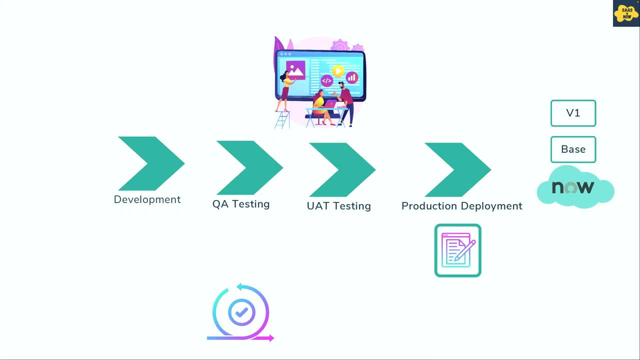 That means that feature is basically moved to production Now. this ensures that all features are working fine in production and performance. Now this ensures that all features are working fine in production and performance with new feature and gives confidence to all the parties involved in the release. 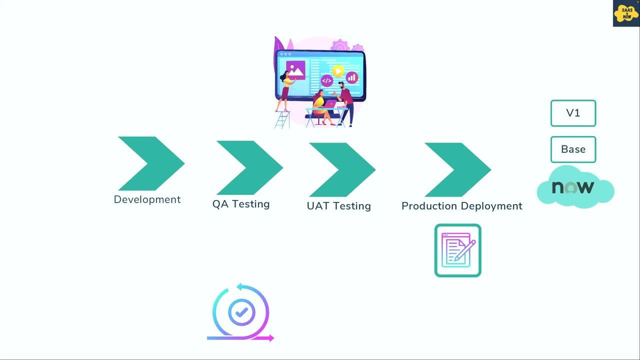 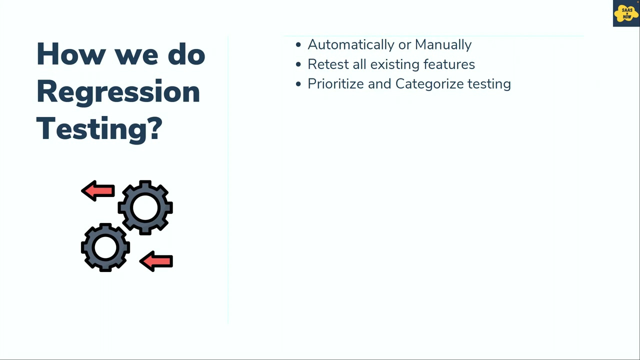 Involvement of regression may vary in different organizations, as some organizations perform regression during UAT and some perform before UAT. So it totally depends on the process of different organizations. Now how do we do regression testing? After multiple releases of a platform or software system, regression testing becomes time consuming. So it's really